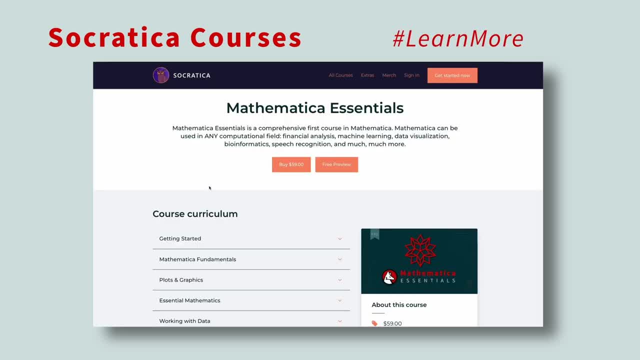 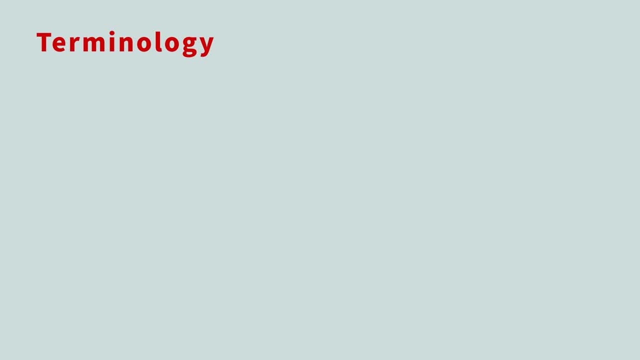 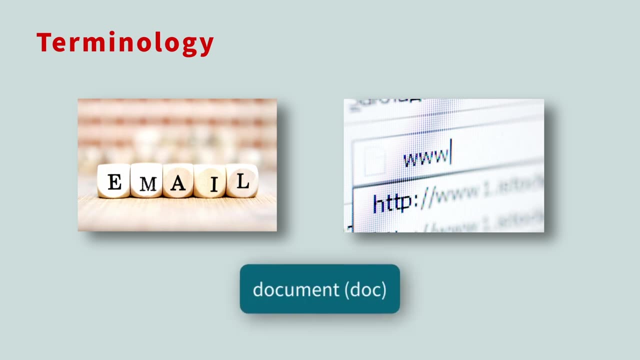 Socraticacom, where you can hashtag LearnMore. Now back to this bag of words. In natural language, processing any text from an email to a web page is called a document, or doc for short. The process of extracting data from these docs is known as feature extraction. 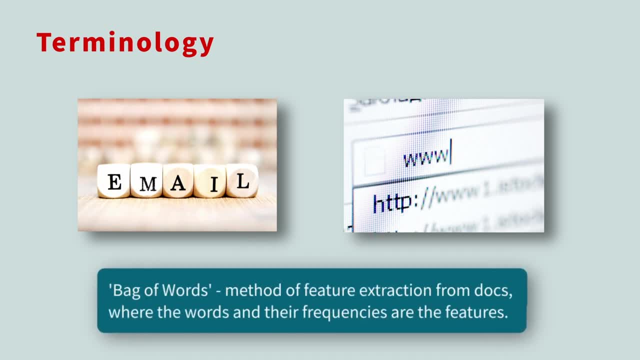 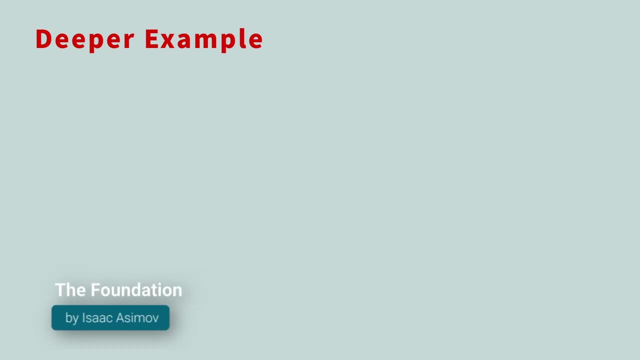 Using this terminology, the bag-of-words model can be described as a method of feature extraction from docs, where the words and their frequencies are the features. Let's create a bag-of-words using an excerpt from The Foundation by Isaac Asimov. 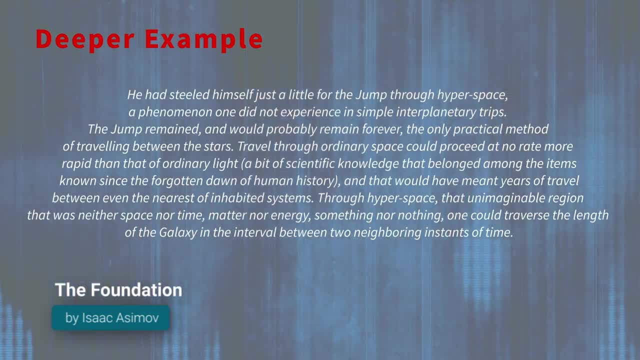 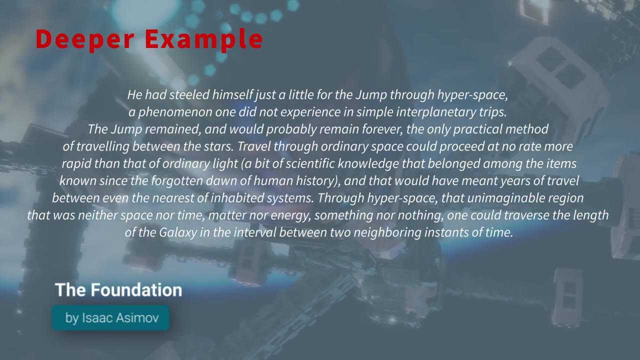 He had steeled himself just a little for the jump through hyperspace, a phenomenon one did not experience in simple interplanetary trips. The jump remained, and would probably remain forever, the only practical method of traveling between the stars. Travel through ordinary space could proceed at no rate more rapid than that of ordinary 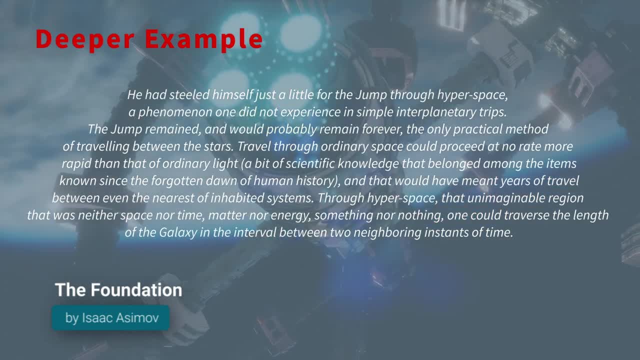 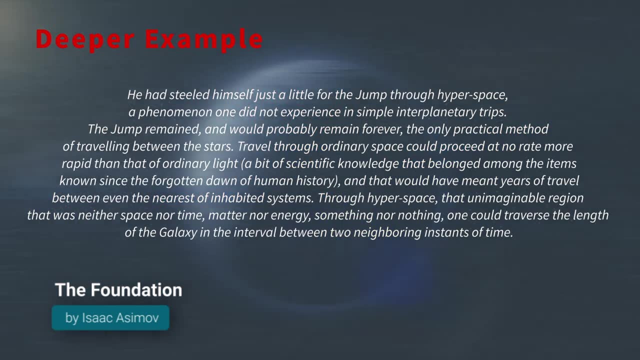 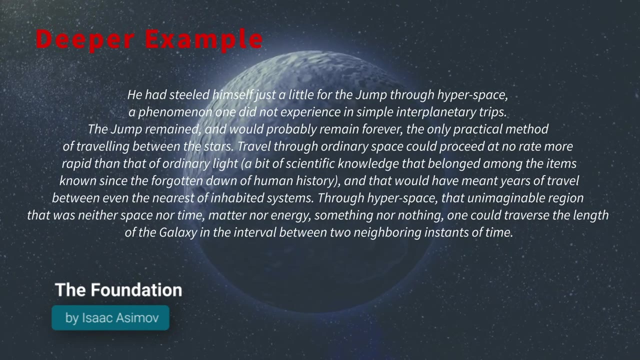 light A bit of scientific knowledge that belonged among the items known since the forgotten dawn of human history And that would have meant years of travel between even the nearest of inhabited systems, Through hyperspace, that unimaginable region that was neither space nor time, matter nor energy, something nor nothing. one could 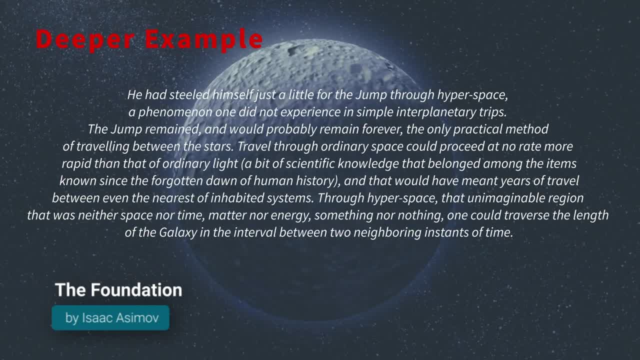 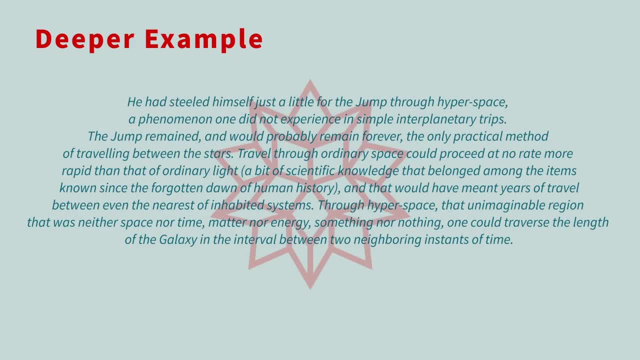 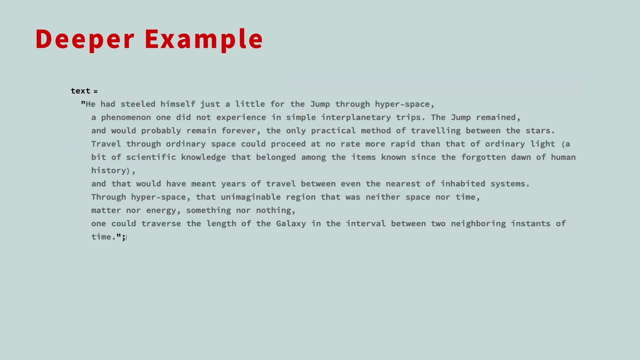 traverse the length of the galaxy in the interval between two neighboring instants of time. We'll start exploring this text using the Wolfram language, known for its long-term readability, especially for those who aren't programmers. Shortly after, we'll demonstrate how to store a bag of words using Python, the most popular language in AI research. 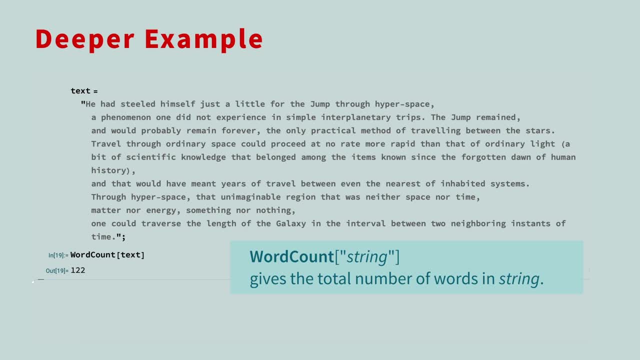 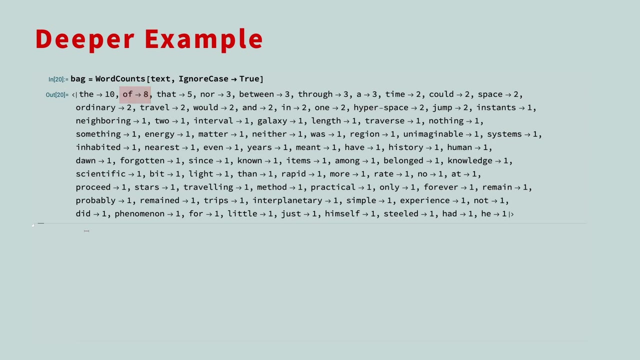 There are 122 words in this text sample. Next, we can look at each word along with the number of times it is used. We will ignore case when counting the words. The word the is used 10 times, Of occurs 8 times, and so on. As you can see, most words were only used once. 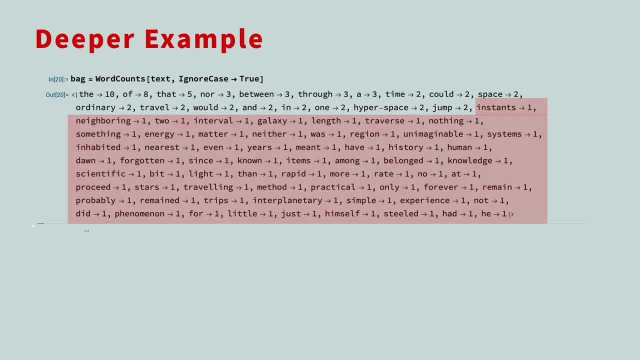 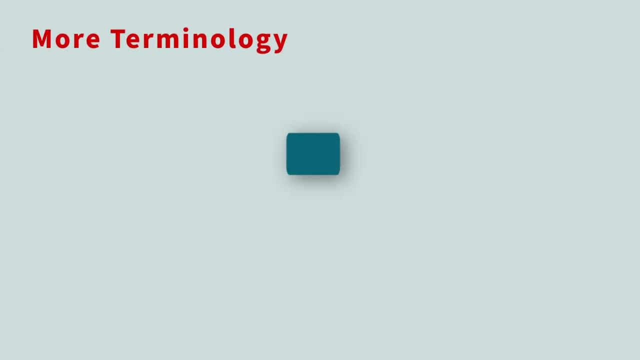 This is common with skilled authors who have a large vocabulary, And if we look at the number of entries in our bag of words, there are only 83 distinct words, So there are 39 words that are repeats. A bag of words is a specific application of a more general idea that's often used to describe. a particular event or event. For example, if we look at a bag of words, we can see that the number of words in the bag of words is the number of words in the bag of words. The number of words in the bag of words is the number of words in the bag of words, The number. of words in the bag of words is the number of words in the bag of words that is used more often in mathematician, specifically discrete math or combinatorics. A set is a collection of items where a word is repeated, and a set is a collection of. 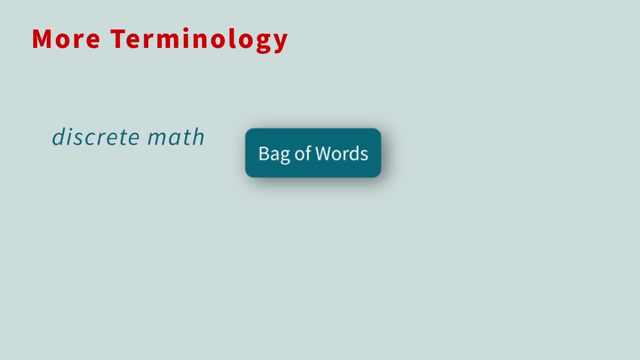 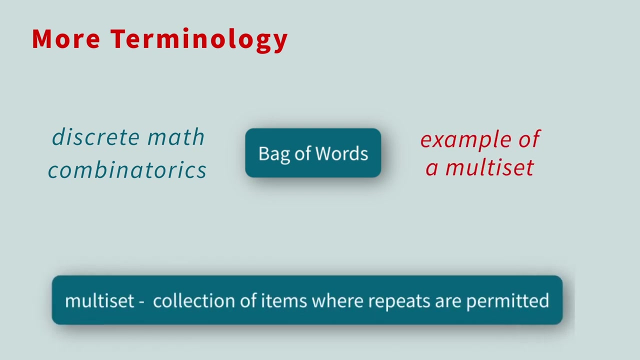 rewards, which isκα repeated words, so that a bag of words contains a tad more computers than any other sentence. But it is an example of a multiset. A multiset is a collection of items where repeats are permitted. If you ever run into a puzzle when working with a bag of words, there is a good chance that mathematicians might need to write this off. So mix it up book to book and then look at the selected numbers. So now what you've seen is the number of words. the killed words are including was from four times 10 or 15.. 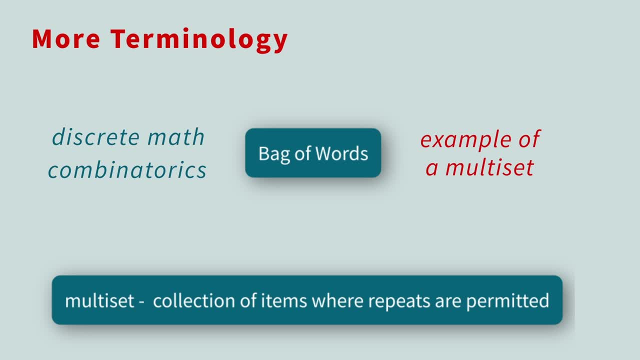 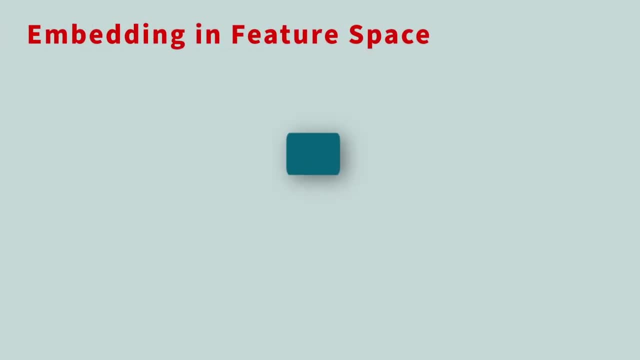 Then see if it was 15, 15.. have already solved it, but you'll need to know these math terms when cracking open that math book. A bag of words is a good first step in extracting features from a piece of text, but it's not the only step. There are still words, and as 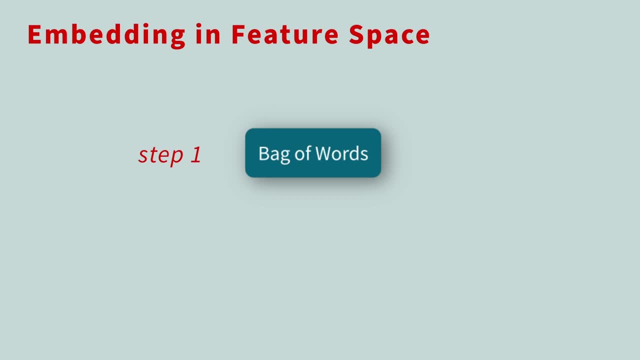 we've mentioned before, computers prefer numbers, So in the next step we're going to convert each bag of words into a vector. Let's see how this is done. Imagine if you took all the words in the English language and then sorted them by. 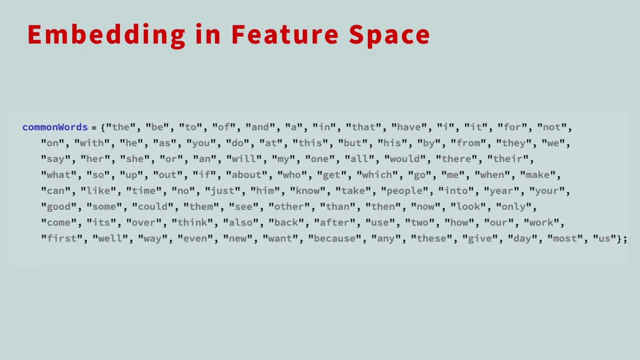 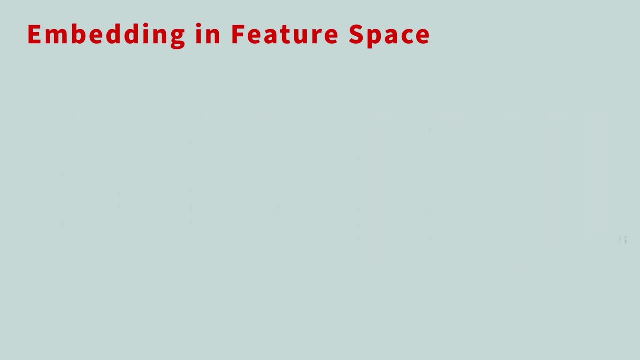 how frequently they were used For a visual. here are the first 100 words, but imagine this list going on and on. To demonstrate the word-removing technique, let's load the text for the book The Adventures of Sherlock Holmes by Sir. 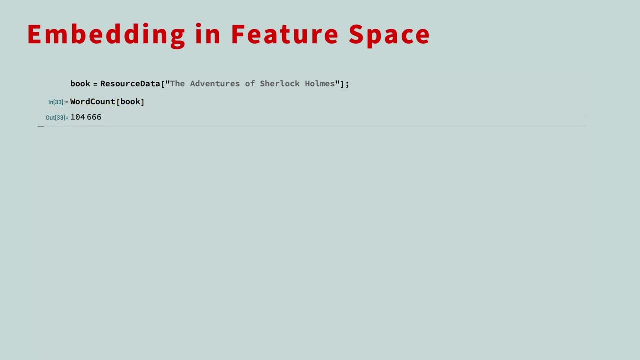 Arthur Conan Doyle. This book has 104,666 words. First, let's construct the bag of words by counting how often each word appears. When we're doing this, we'll ignore letter case. For the next step, we'll take the list of the 100 most commonly used words and replace each 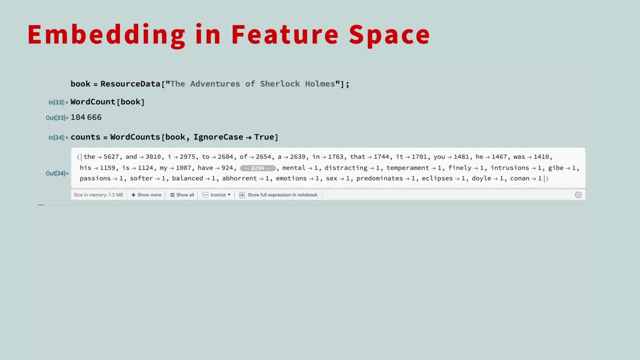 word with how often it occurs in the book. If we look up how many times the appears, we get 5,627.. The next word, be, occurs 627 times. To is used 2,684 times, and so on. If you do this for. 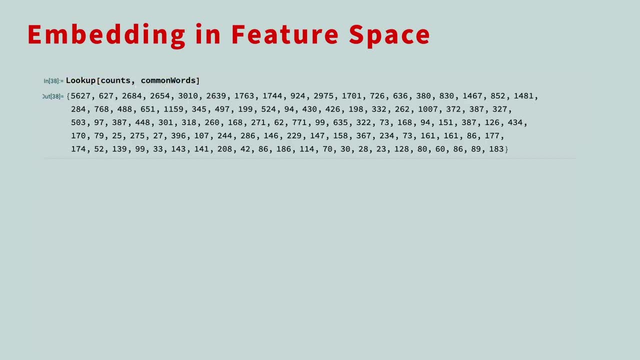 the words, you get a sequence of numbers. Here we're only showing the first 100 numbers, but you could compute this for the entire English dictionary. This sequence of numbers is a vector and it lives in vector space The length of the. 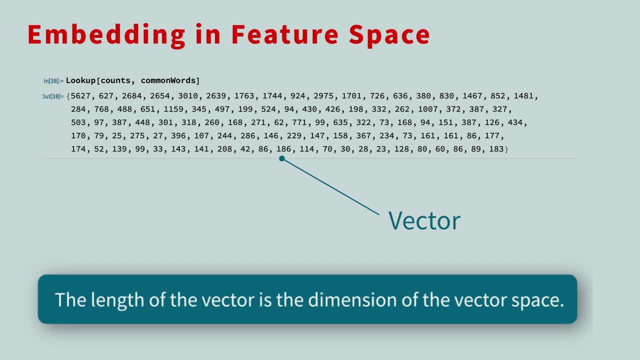 vector is the dimension of the vector space. This shortened example is a vector in 100-dimensional space, but in practice you would use many more words, which means a much higher dimension. In natural language processing you will often refer to this vector space as feature space, since the numbers and 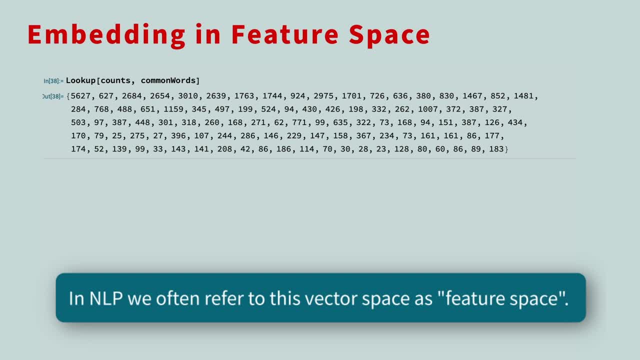 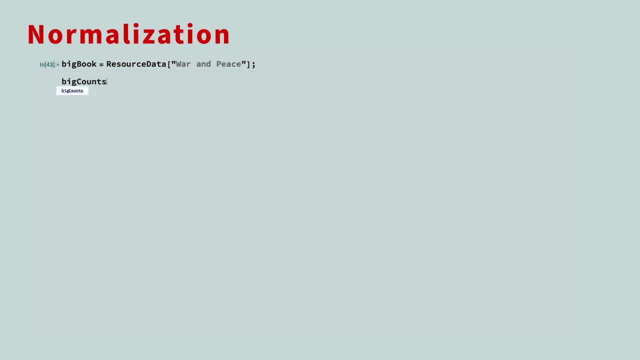 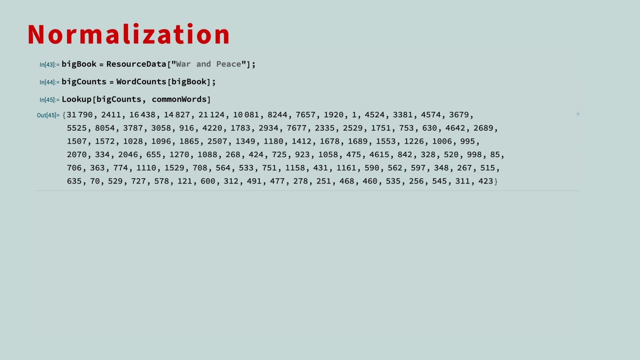 vectors are features extracted from text. Let's look at the feature vector for a much longer book: War and Peace. As you can see, each number in this vector is many times larger than for Sherlock Holmes. This can compel things, because larger documents inherently have higher word counts To. 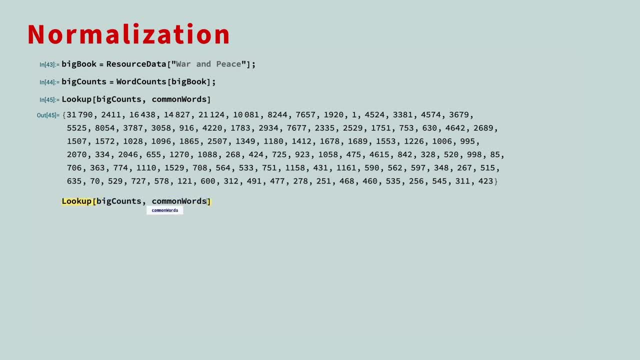 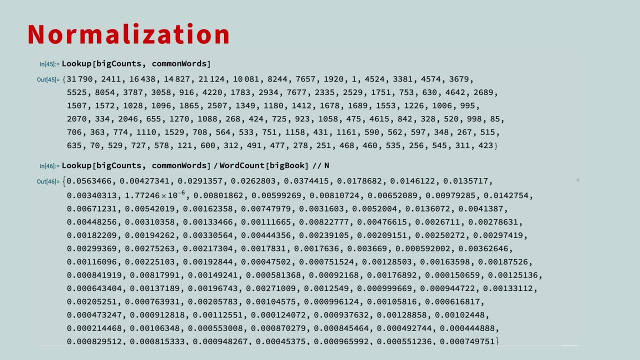 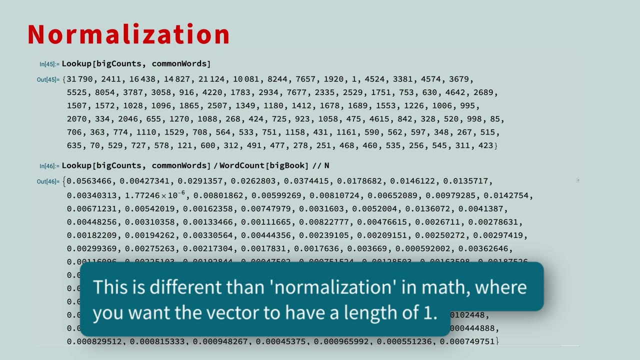 address this. a simple yet effective approach is to divide each number in the feature vector by the total number of words in the document. This technique, called normalization, adjusts for the document length and allows for more meaningful comparisons between docs of different sizes. We've seen how you can. 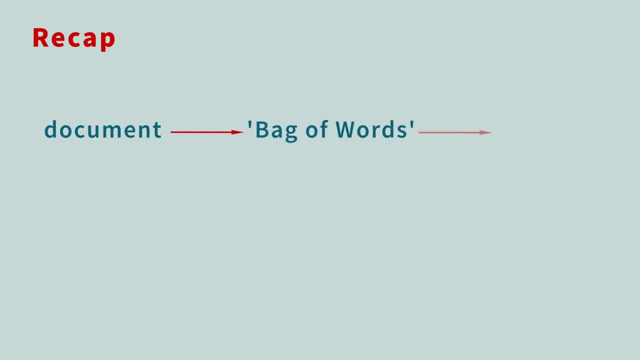 take a doc, convert it to a bag of words, then turn this into a vector inside feature space. Normalization is a helpful step before you start training your machine learning algorithms. In upcoming lessons we'll learn about similar techniques like TF-IDF, which stands for Term Frequency, Inverse Doc Frequency. So 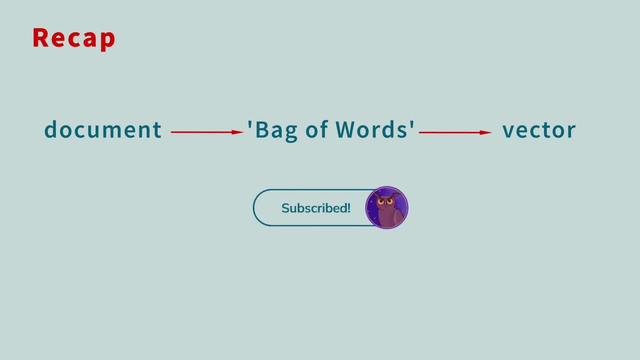 be sure to put Socratica into your bag of subscribed channels. you